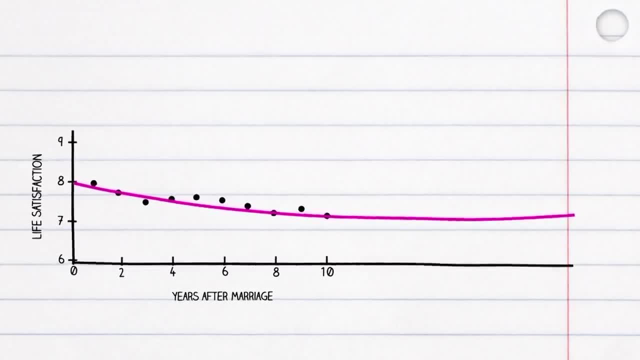 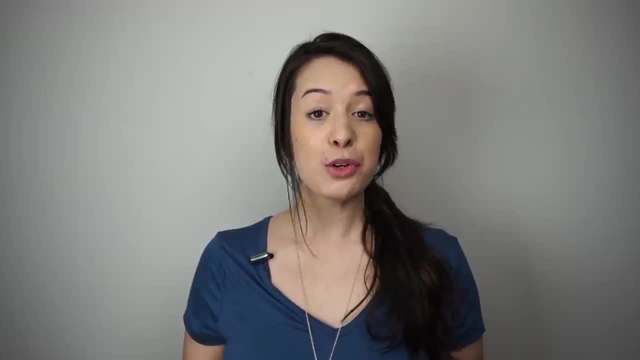 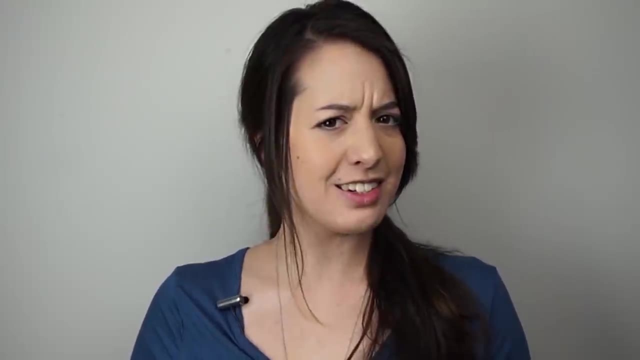 and the trend seems to align more with what psychologists say, That there's a slight comedown after the honeymoon bliss, but that life satisfaction more or less levels out over time. So if using two factors is more accurate than using one, adding more information should lead to a more accurate prediction, right. 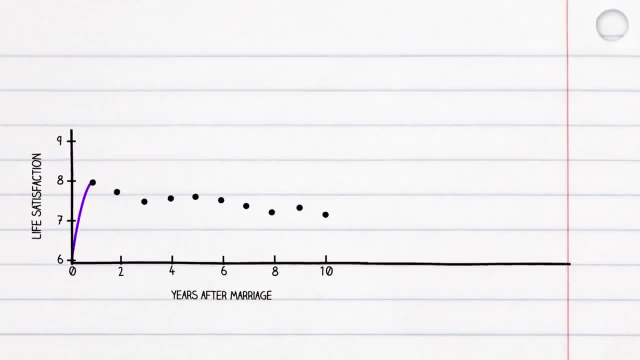 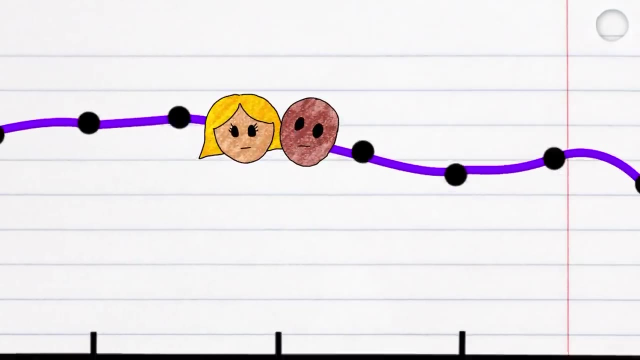 Well, let's try it with nine factors. It does a good job of modelling the current data as it fits through every point, But it misses the overall trend. It shows that couples are deeply miserable right up till their wedding day. Their marriage is then a series of severe ups and downs, and after 10 years they 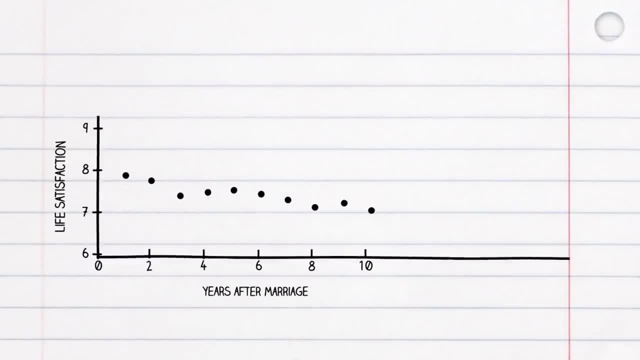 drop into a sudden deep depression. What's more, if the same study were repeated with different couples, the inevitable slight variations in data would have a huge impact on the nine-factor prediction, But it would leave the two-factor model pretty much unchanged In practice, obscuring data. 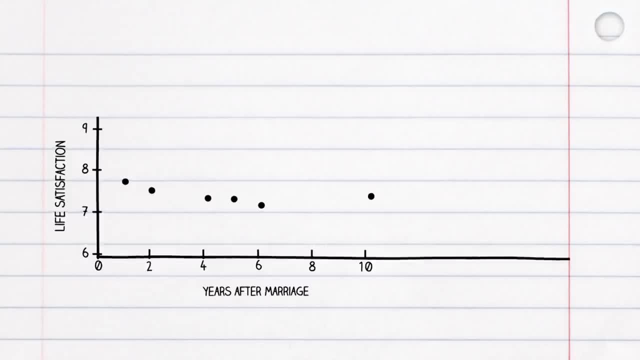 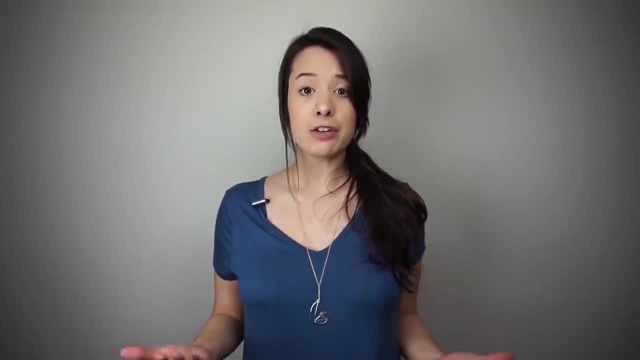 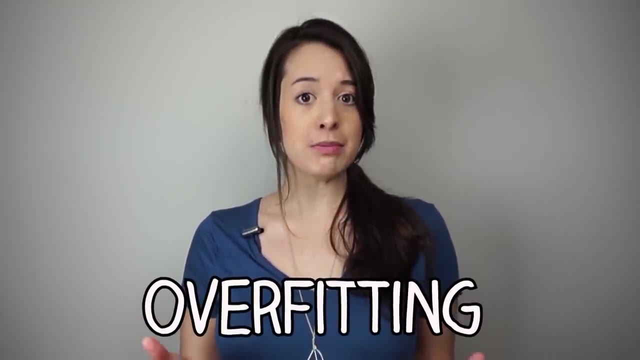 adding random noise or withholding information often makes for better predictions. By placing too much emphasis on each individual data point, we lose sight of what's really important – the trend. This idea is called overfitting, and it tells us that sometimes. 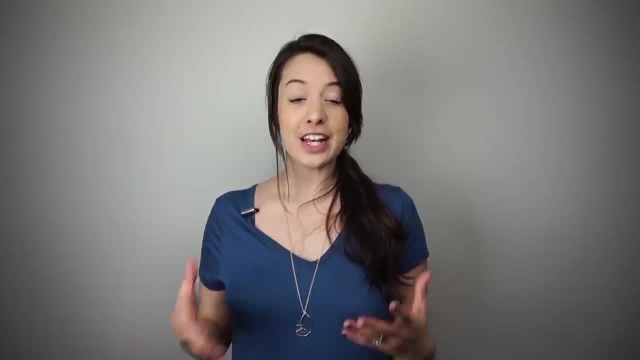 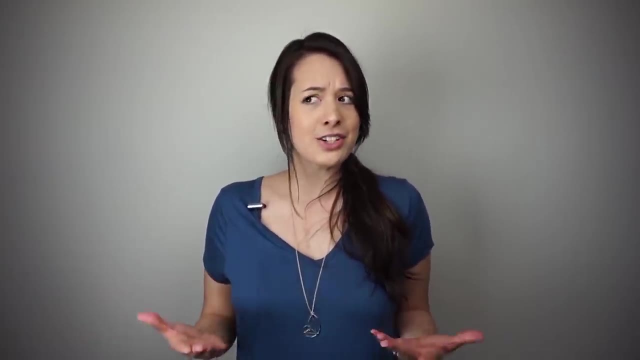 the less we think, the better off. we are Overfitting, and the wrong predictions it causes are usually results of placing too much emphasis on what we can measure, while forgetting what's actually important. I know this all too well from my high school and university days. I was always working to get a 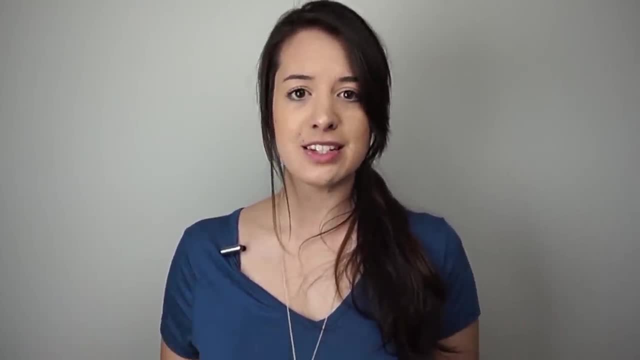 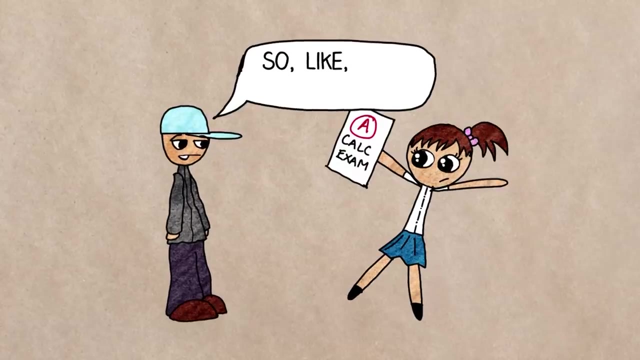 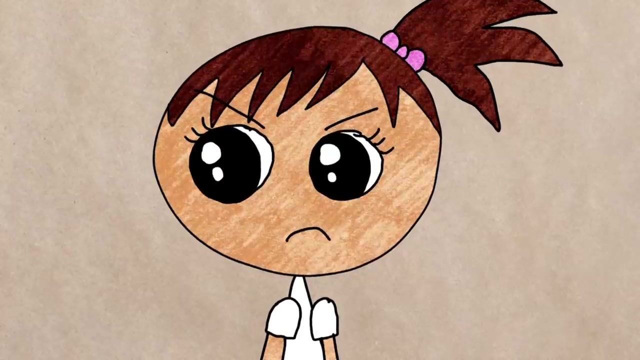 good grade, while not really trying to get a deep understanding of the actual subject matter. I'd get an A on a calculus exam, but if my brother asked me So, like what is calculus? Well, I'd have no idea. 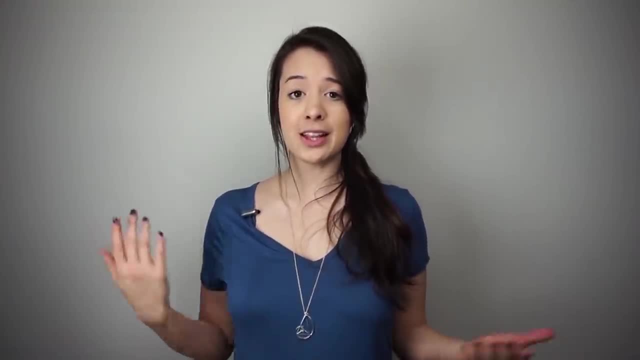 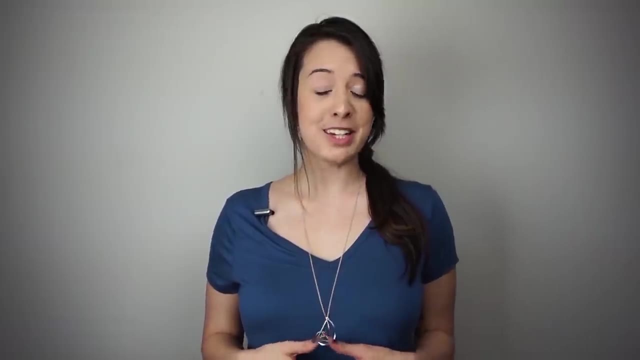 I was paying too much attention to what I could measure, consequently missing out on actual learning. Classic overfitting. But overfitting isn't just in the schoolyard – it's in our biology. Our taste buds were designed to help us detect which foods are healthy. 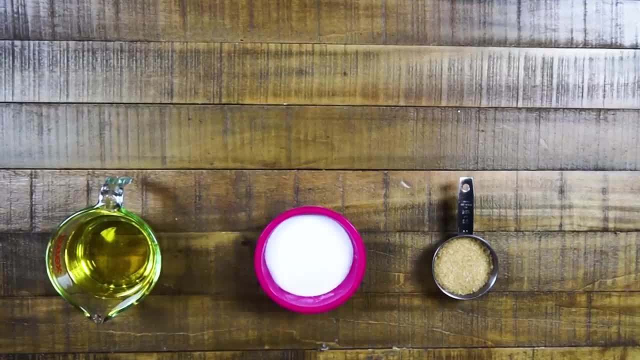 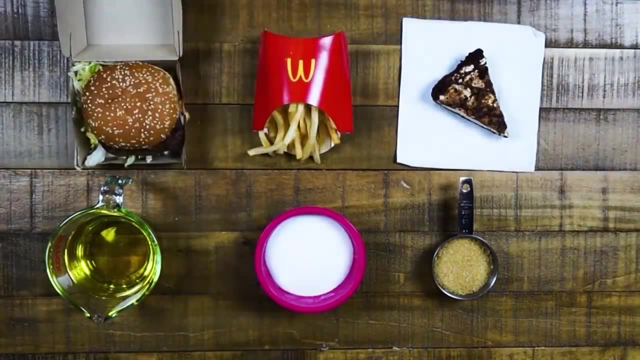 Sugar, salt and fat are all essential parts of our diet, so it makes sense that we're programmed to think they taste good. But since we started modifying our food to contain unnatural and unhealthy amounts of these ingredients, taste has stopped serving as an accurate guide to what's healthy. 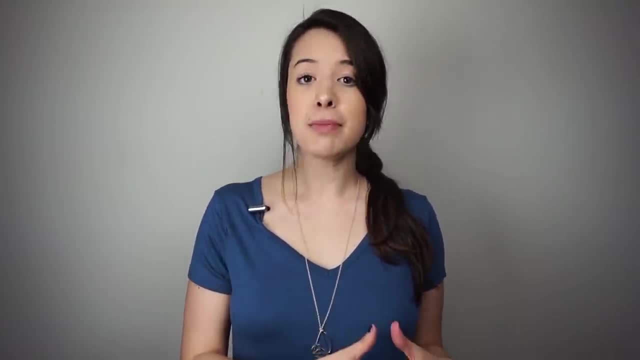 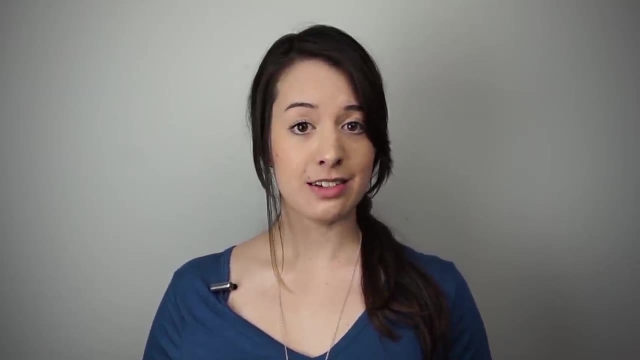 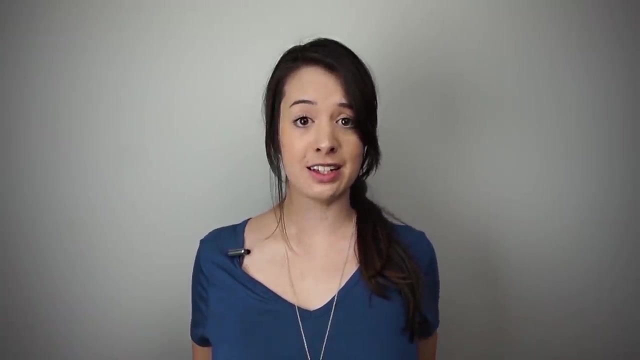 Our brains are overfitting for an outdated metric optimising for taste instead of what taste is supposed to provide – health, As economist Charles Goodhart said. So what can we do about overfitting? Well, in machine learning, there's a technique called regularization. 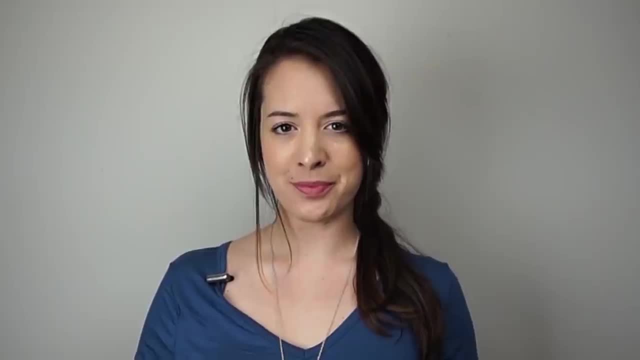 which can be thought of as a kind of complexity penalty. For example, one method of regularization is to scale down the weight of food. That means to do the same thing over and over. One method of regularization is to scale down the weight of food. 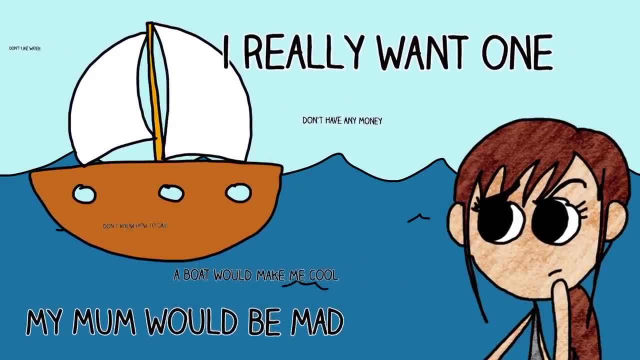 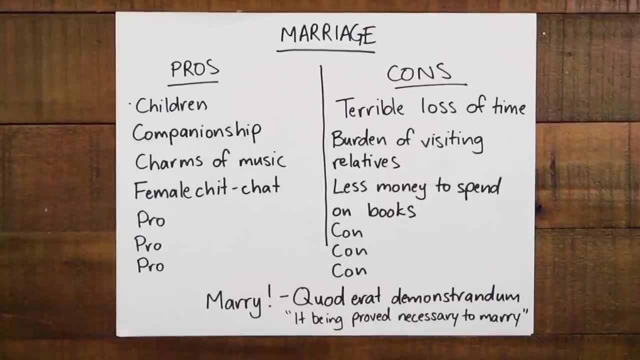 down the weights of all the factors until most of them are at completely zero. this means that only the most important few have any say in the final decision. in darwin's situation, this might have looked something like crossing out the less important stuff, like children and companionship. 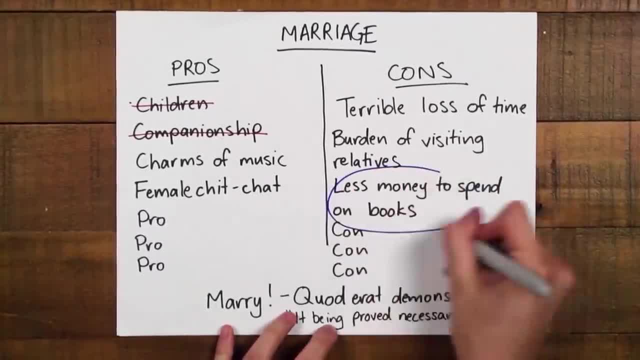 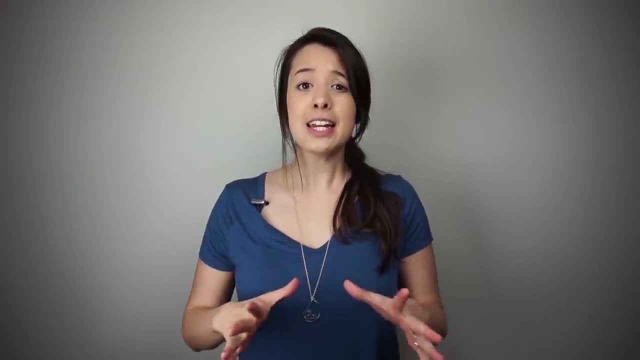 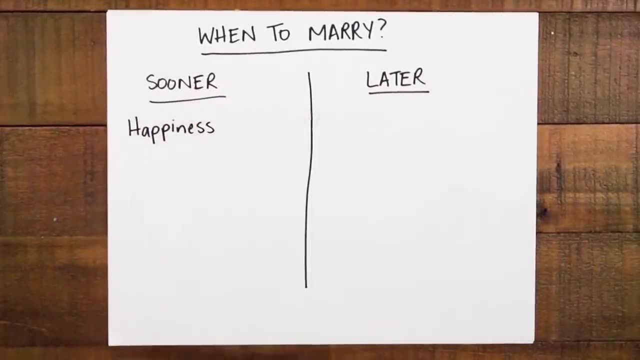 and keeping only the stuff that really mattered, like not being able to spend as much on books. speaking of darwin: right after he decided to marry by proof, he immediately started fretting about when to marry. he wrote yet another list of pros and cons, considering things like happiness. 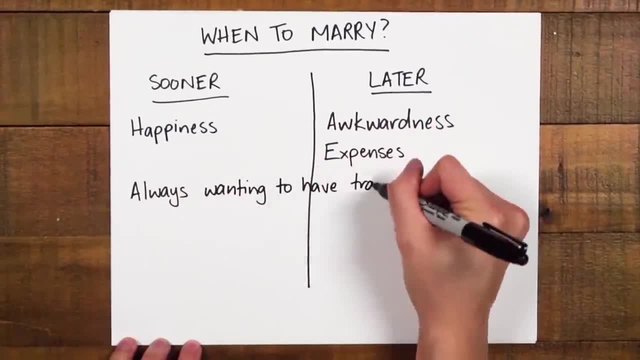 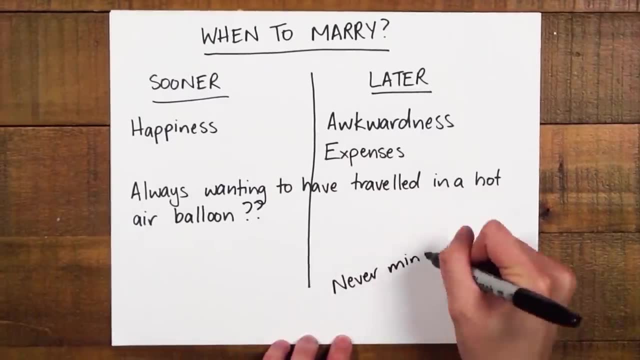 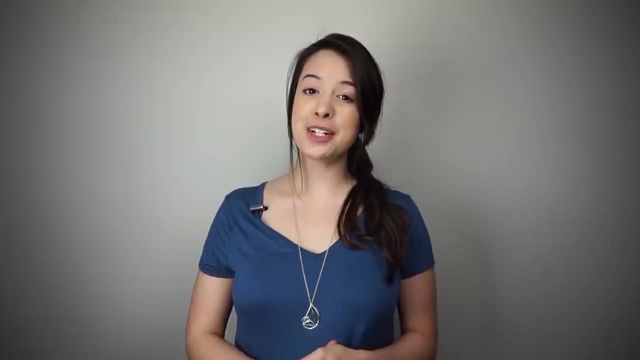 awkwardness expenses, always wanting to have traveled in a hot air balloon. not sure whether that was a pro or a con, but by the end of the page he resolved to never mind trust. to chance, he had his own methods of regularizing. he married emma wedgwood and they lived happily ever after. 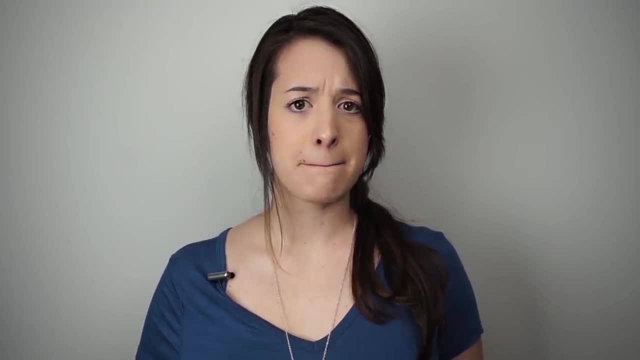 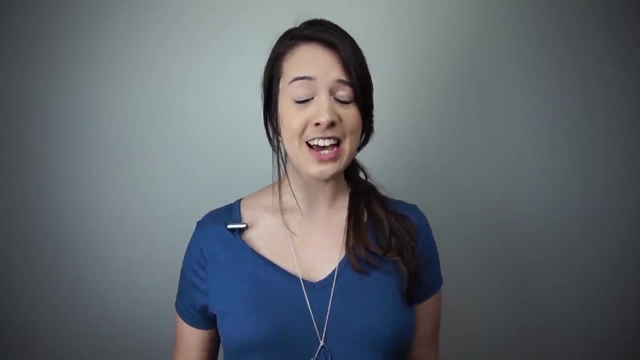 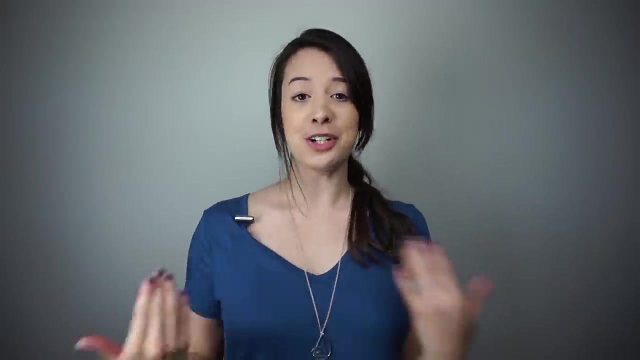 until he died of congestive heart failure at 73.. thanks for watching, guys. so i hope this video helped you out in some way. if you're prone to overthinking, i know i definitely am. um, even while i was making this video, i usually like fret about what to leave in and what to leave out and what you guys are gonna like. 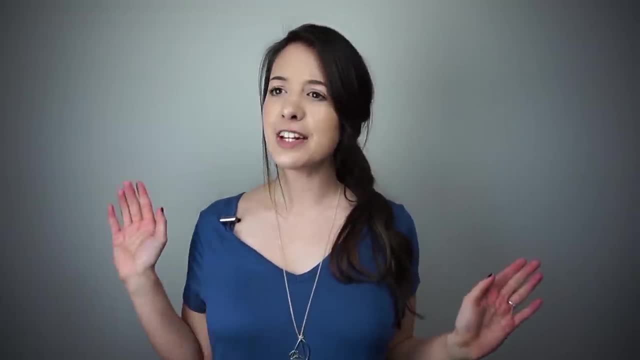 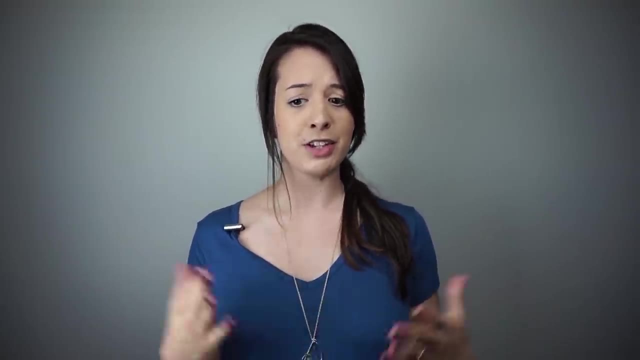 and in the spirit of not overfitting, i just thought: for this video, i'm just gonna go with my first instinct and i had a lot more fun, so i hope that you can get something out of this video too, and if you're lucky enough to like not be an over thinker, share it with someone who is oh and i. 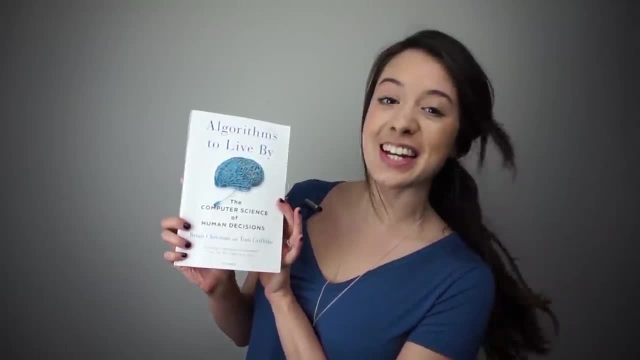 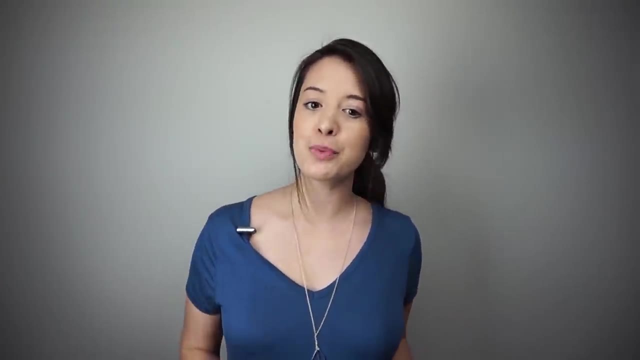 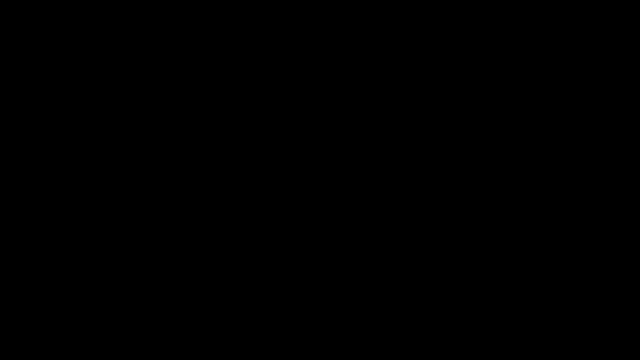 also want to mention that this video was based on this amazing, amazing, amazing book algorithms to live by by brian christian and tom griffiths. i've done a few videos based on this book which i'll leave for you guys in a playlist at the end on the end screen. um yeah, until the next video, bye. bye.